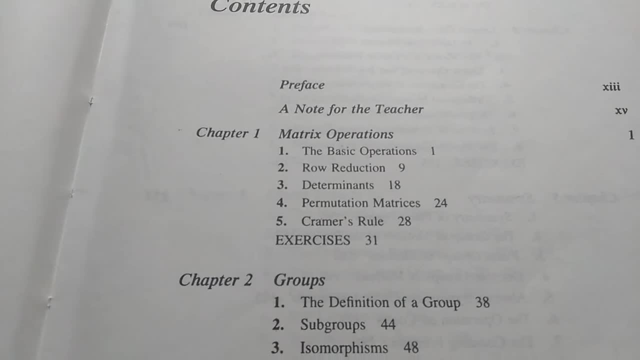 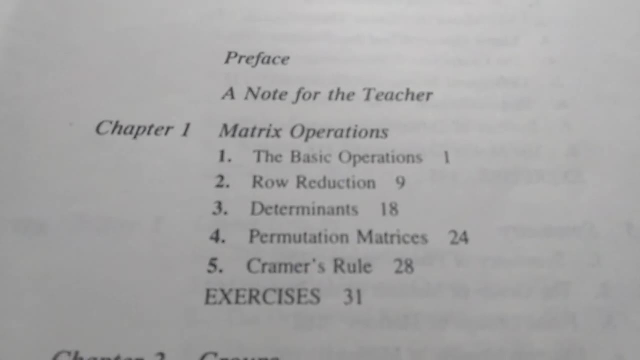 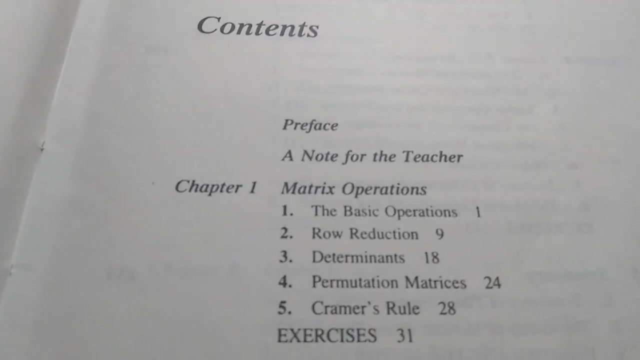 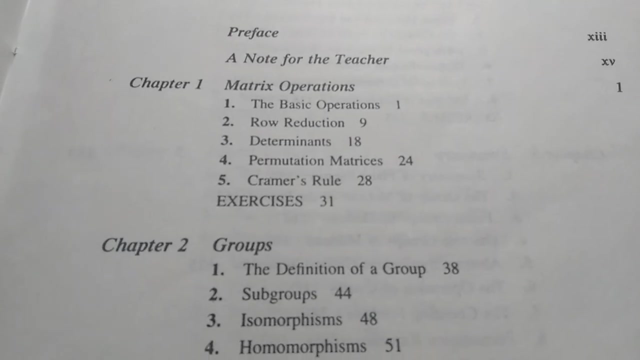 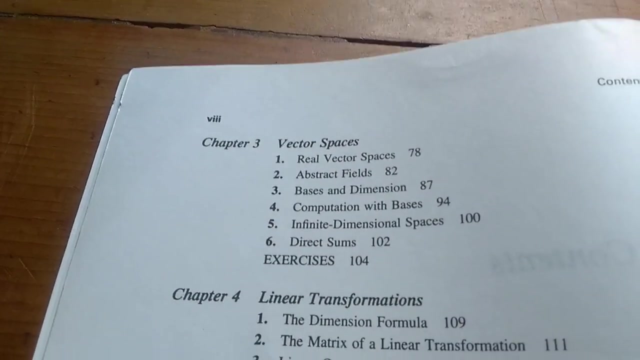 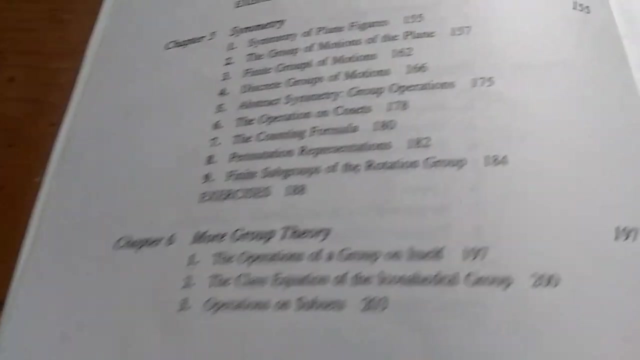 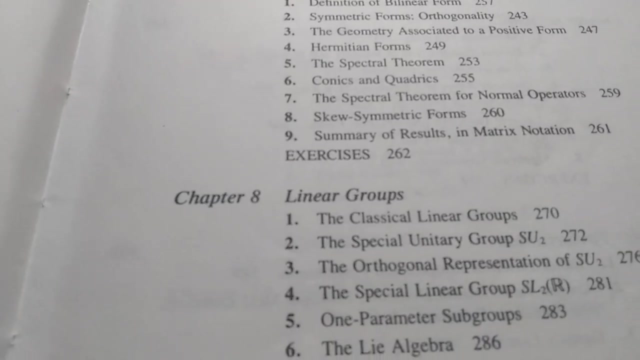 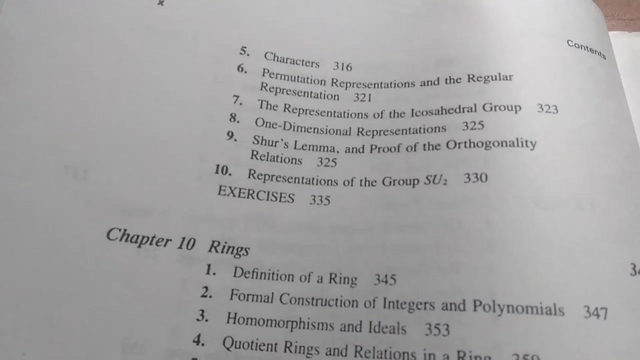 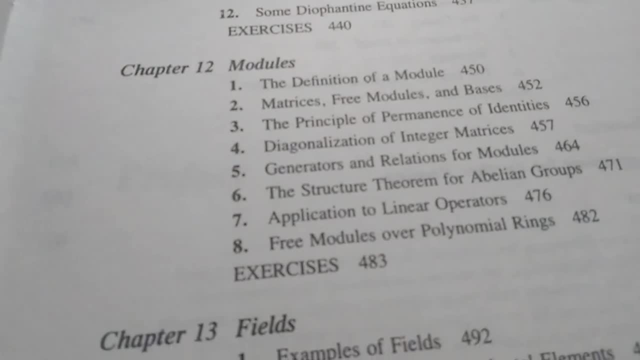 It's completely different, right? It's a completely different setup. I think it's because he starts with linear algebra. That's what makes it so different. Also, the writing style of the author 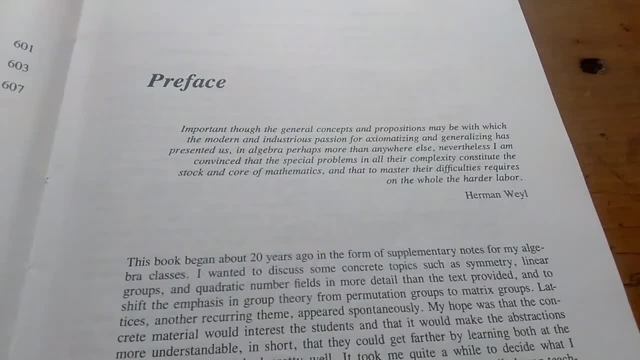 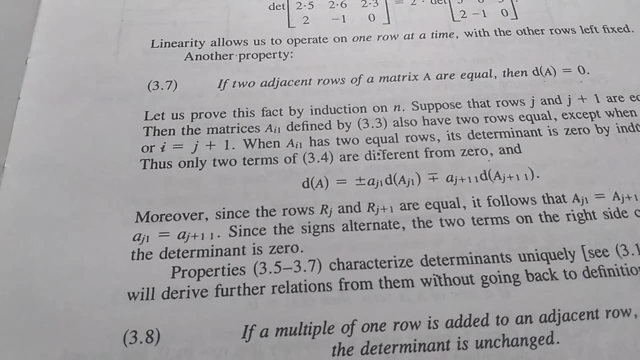 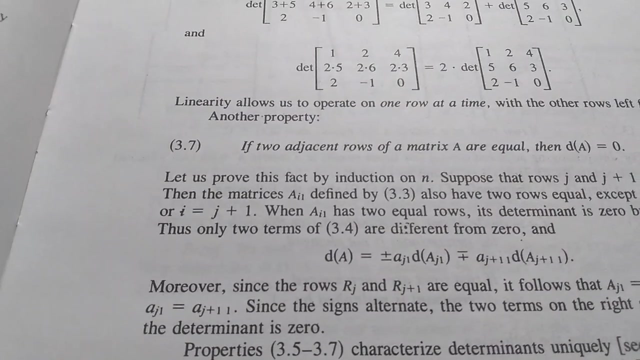 is completely different. Let's talk more about that. So Michael does an excellent job writing this book. It's just written so well compared to other algebra books. If you're looking for a book to read and learn from, this is a good one. That is one of the pros of this book. 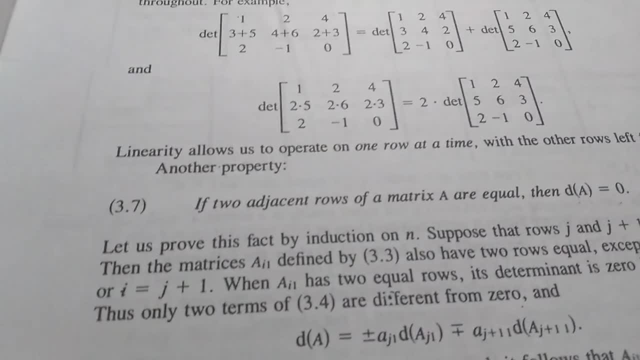 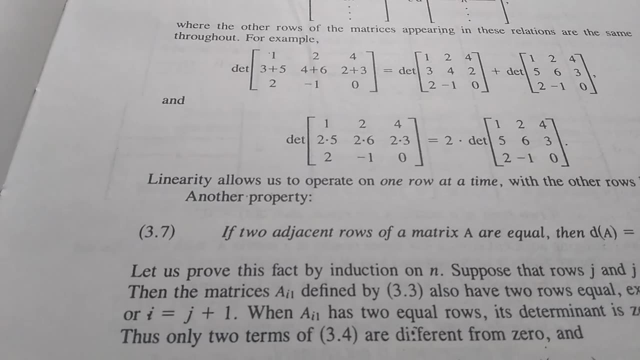 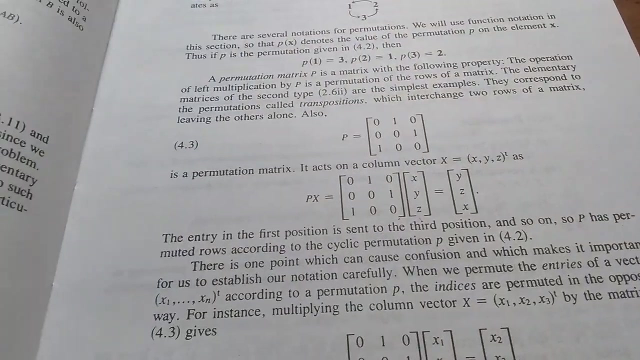 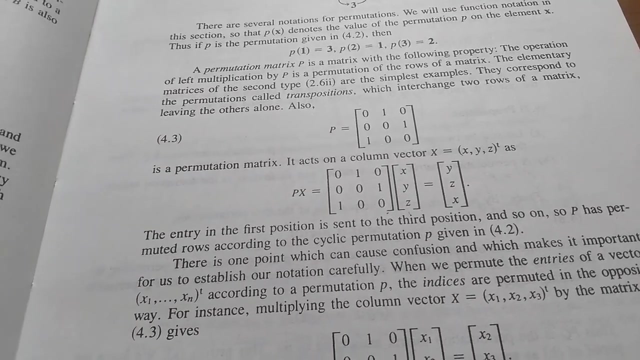 Now, there are some cons, and I think the biggest con of this book is that it's hard to use this as a reference. I found that whenever I was trying to look something up in this book, I had a hard time finding it. I don't know if the index is not sorted in a good way or it's just a non-standard book, but I had a hard time finding things in this book when I needed them. So it's a good book to read and learn from, but I don't think it's the best reference book out there.